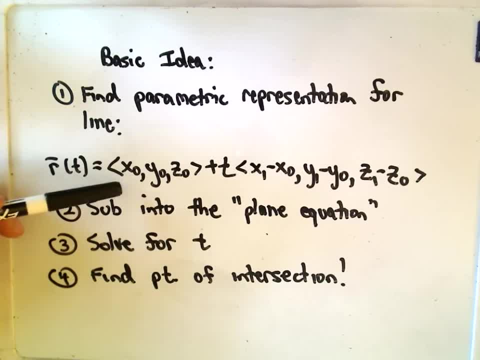 So you take one of the points on the line and you use the position vector that would point at that line, And then we find the direction vector that would go through the two points. Multiply that by t. We can put that together. That will give us the parametric representation. 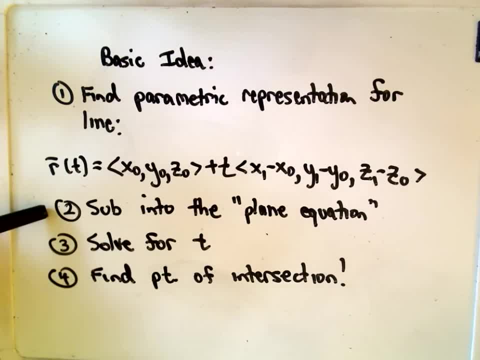 We then just take each of those, We'll substitute that stuff into our plane equation, We'll solve for t And then we'll backtrack and that will help us find our point of intersection. So what do I mean here by all of this? 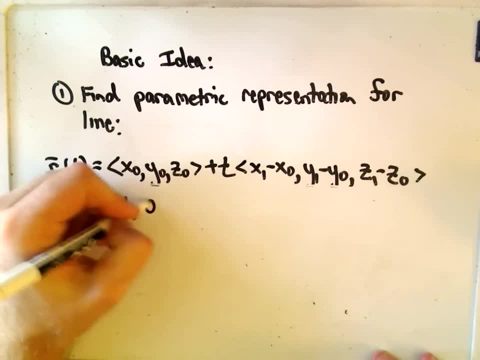 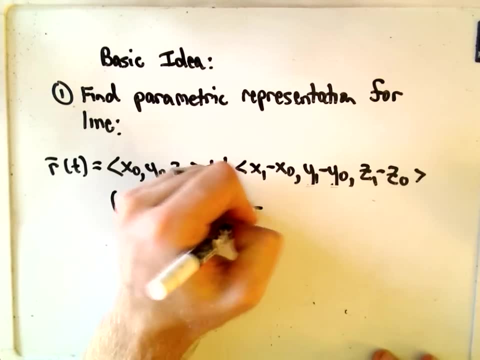 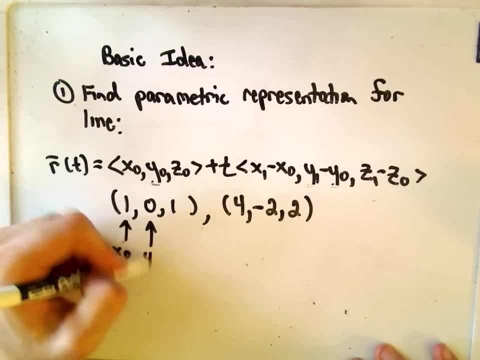 Well, again, we had our point 1,, 0,, 1.. Let me just label these first, So 1,, 0,, 1.. And we had this point 4, negative, 2, positive, 2.. Okay, so, this will be my x naught, my y naught. 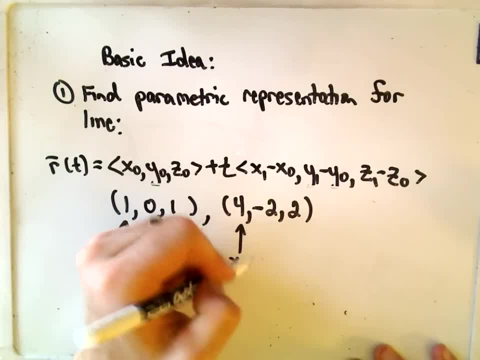 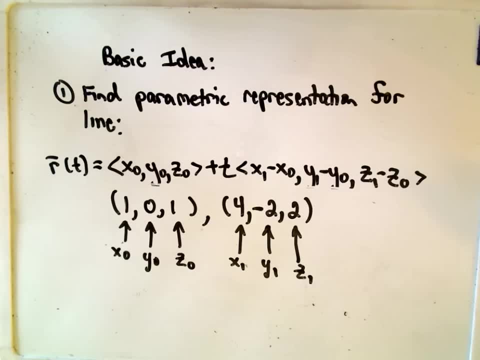 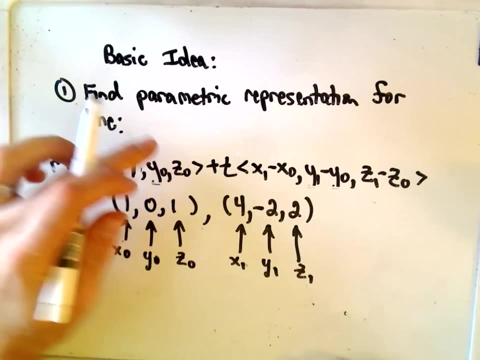 And my z naught. sorry, This will be my x1,, my y1, and my z1.. So again, now it's just a matter of plugging all these values into this equation. So x naught is 1, y naught would be 0, our z naught is also 1.. 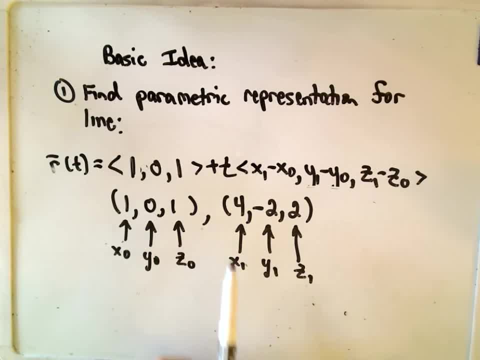 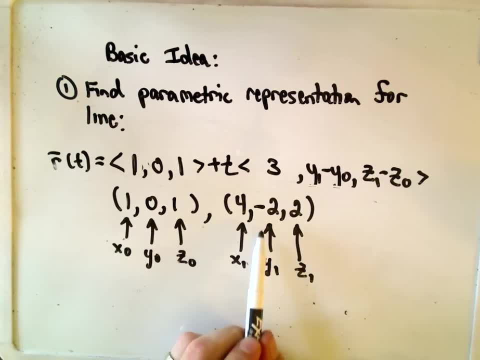 We leave the t alone, And then we simply have to subtract them. So I'm going to do this. So we would take 4 minus 1. That would give us 3.. We would take negative 2 minus 0. So that will just give us negative 2.. 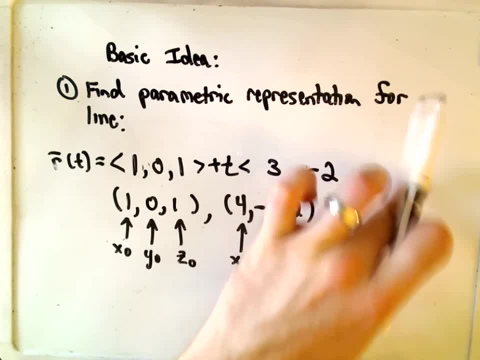 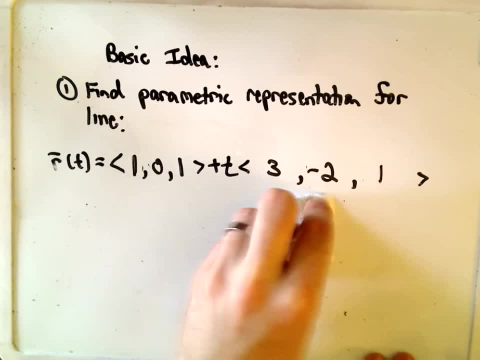 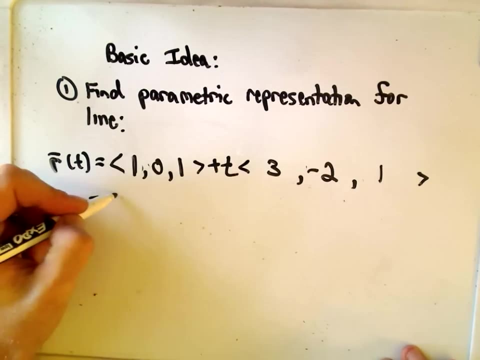 And then we would take 2 minus 1. Which would simply give us 1.. So let's clean this up, make it look a little bit prettier. Okay, so we could write this again: We distribute the t and then we add respective components. 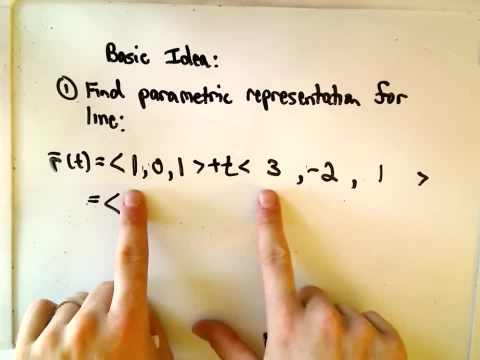 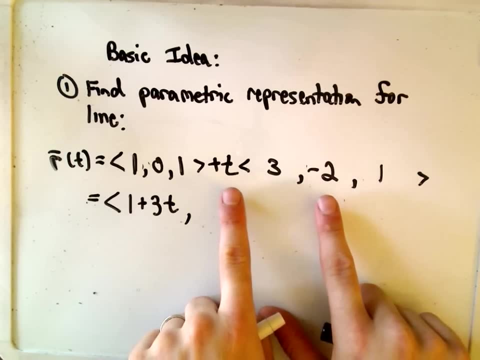 So we would get t times 3. Which is 3t. And then if we add the first components, well, we would simply get 1 plus 3t. If we do that for the middle component, we would get negative 2t plus 0.. 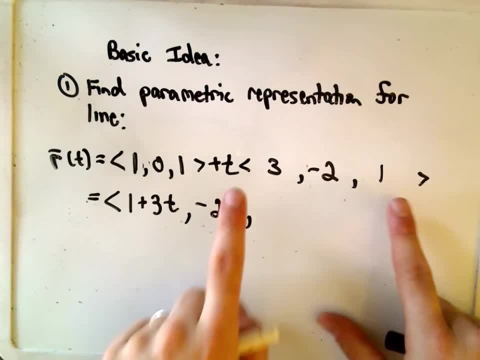 Which is simply negative 2t, And then we would get t times 1 plus 1. Which would just be t plus 1.. So now we have our parametric representation of the line And remember, the first part is a representation for the second part. 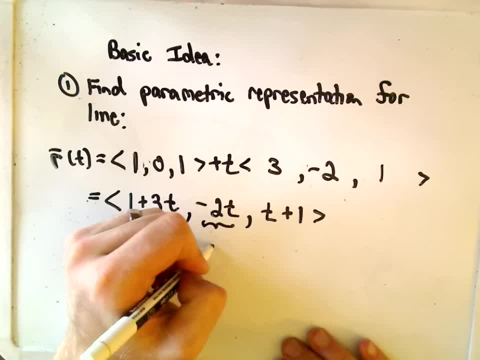 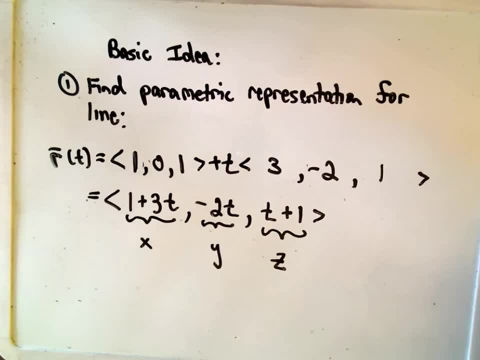 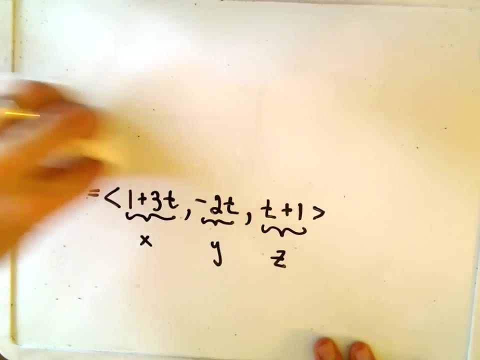 It's a representation for the x coordinate, The second part is a representation for the y coordinate And the third part is simply a representation for the z coordinate. Okay, so we've done that. Now we just need to think about our equation of our plane. 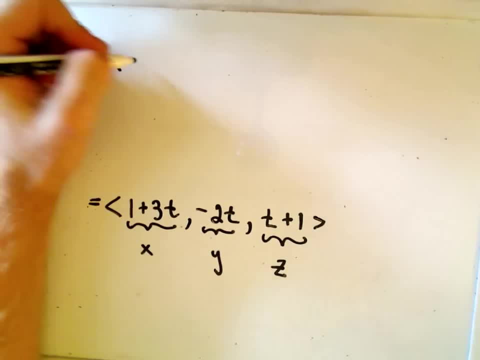 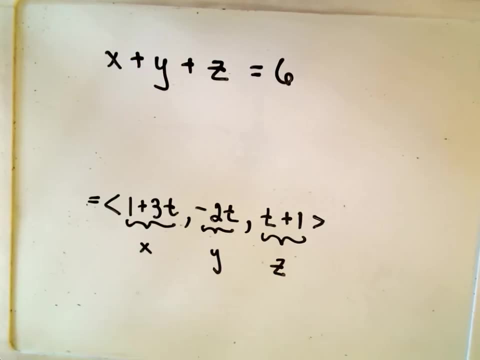 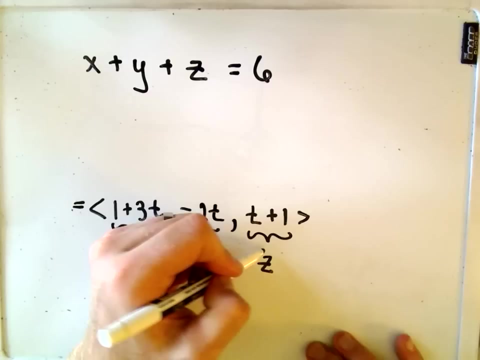 Well, the equation of the plane that we wanted to intersect was simply: x plus y plus z equals 6. And now all we have to do is we simply substitute in our respective x, y and z values. This will give us an equation involving only t. 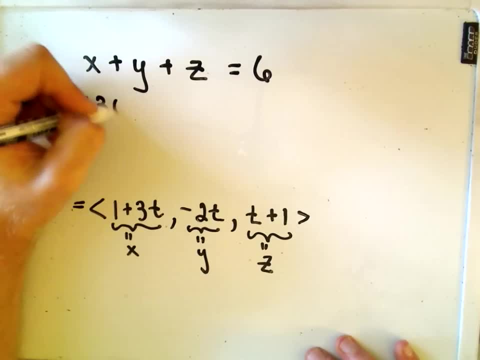 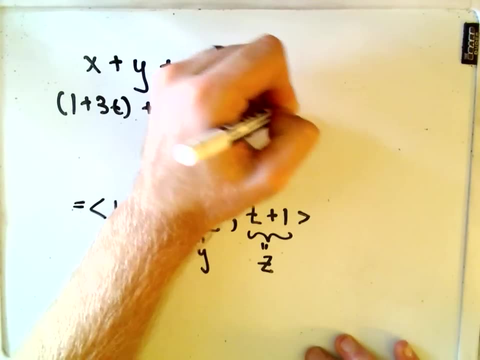 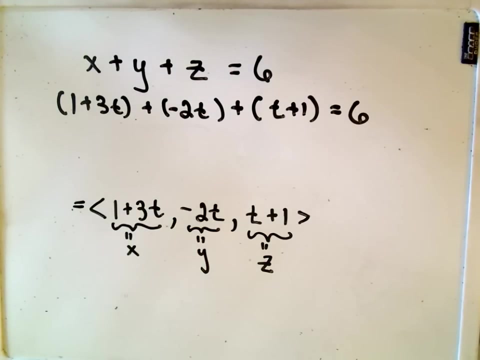 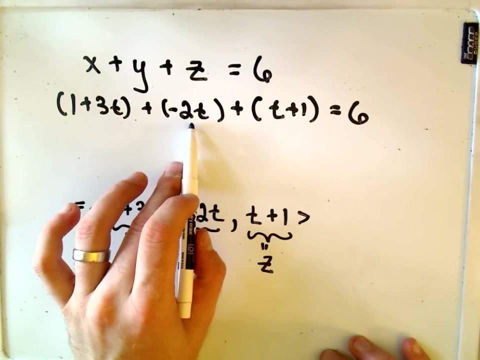 And then we'll figure out t. So we would get 1 plus 3t plus negative. 2t plus t plus 1 equals 6.. Okay, so let's see if we can manage the arithmetic here. So 3t minus 2t, that would be 1t. 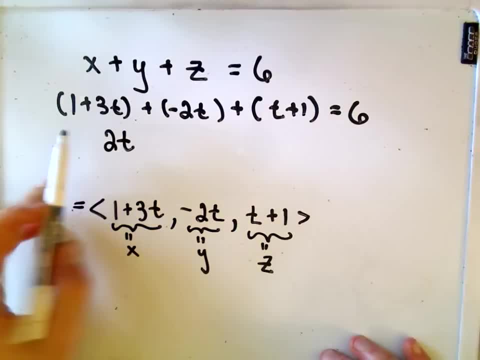 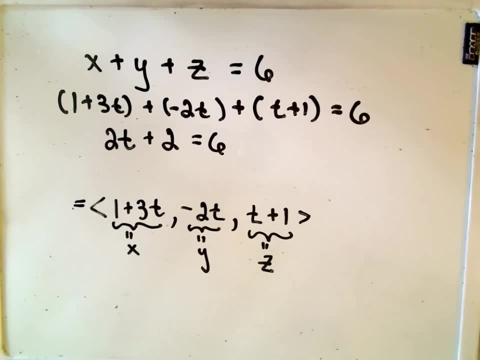 1t plus t would be 2t. We have 1 plus 1,, so that looks like 2, equals 6. And if we simply subtract the 2,, we'll get 2t equals 4.. Divide by 2,, we'll simply get t equals 2.. 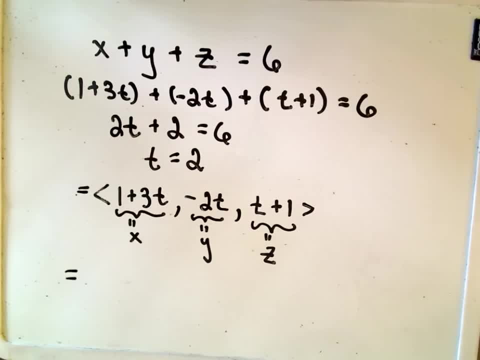 And now all we have to do is simply just backtrack. And now all we have to do is simply just backtrack. And now all we have to do is simply just backtrack And plug these into our parametric equations. And it says the point of intersection. 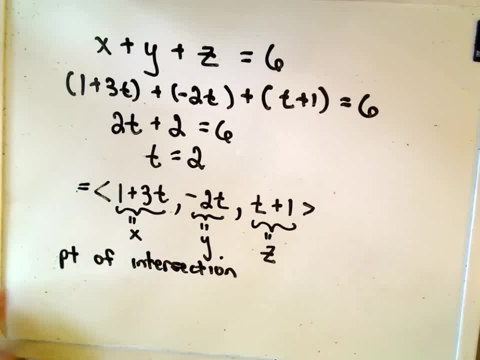 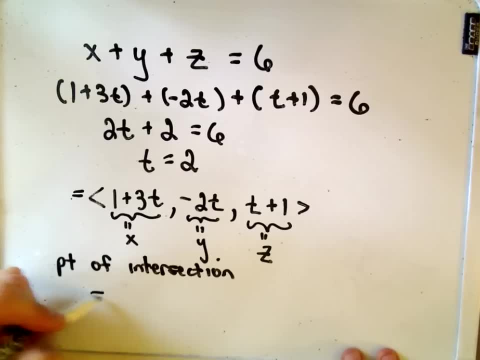 So the point of intersection? it says the line is going to hit this plane at the value when t equals 2.. So if we simply plug that in, that's going to give us the point. Okay, so we would get 1 plus 3 times 2..